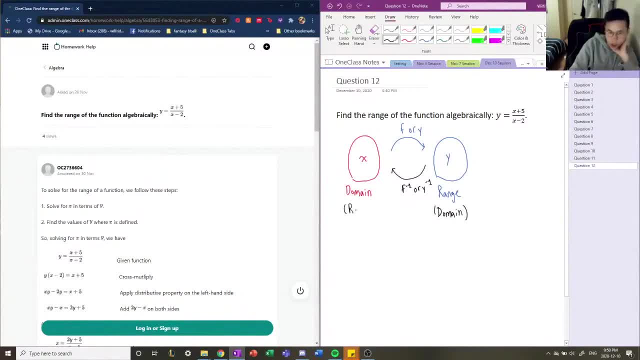 function is going to be the range and the range or the domain of the original function. the range of the inverse function is going to be the domain of the original function. That makes sense, okay. So a strategy that can be involved to calculating the ranges of original functions is to find: 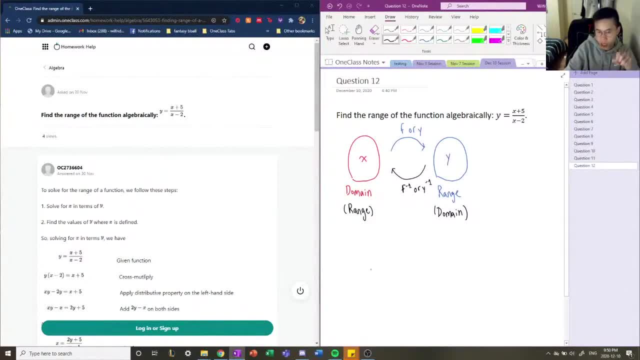 the inverse function and then find its domain. Once you find the domain, then it's equal to its range. Another strategy is that you can just look at and evaluate the nature of the function itself and come to a logical standpoint of what the range is, Or you can just graph. 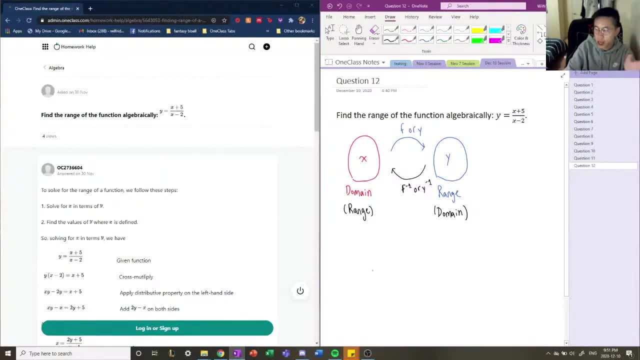 it out and see where the range lies. okay, But we're going to use this inverse strategy because it is the most I guess it covers. we don't really need to use our rationale, or we don't need a graph, right? So it's kind. 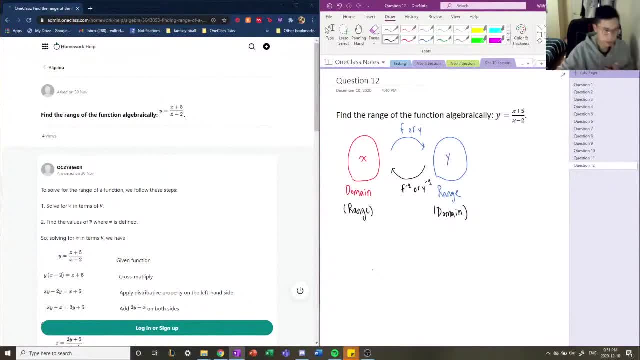 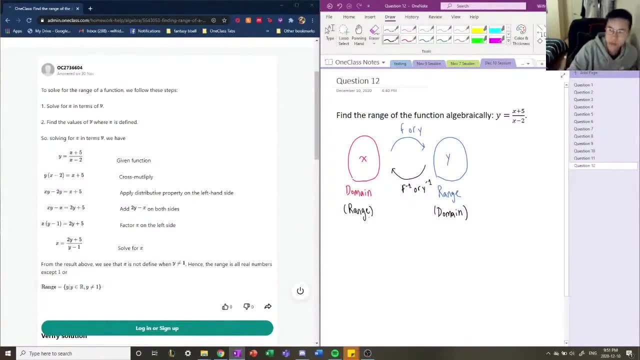 of the easiest way. Okay, so we have our function here: x plus 5, divided by x minus 2.. Okay, so we're going to isolate for x. okay, So, if you're going to isolate for x, then we're going to first of all cross multiply. 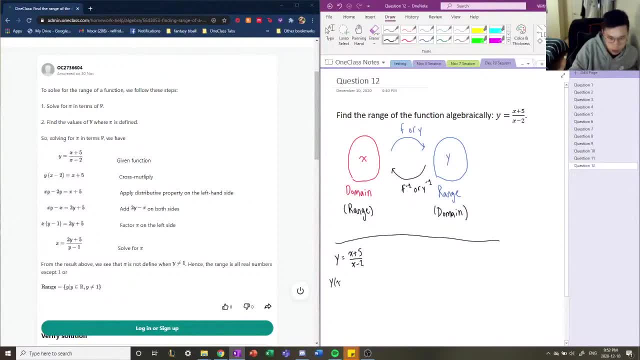 So we're going to multiply both sides by x minus 2.. So we get x minus 2 times y equals x plus 5, okay, If we expand, we get x times y minus 2y equals x plus 5.. Okay. 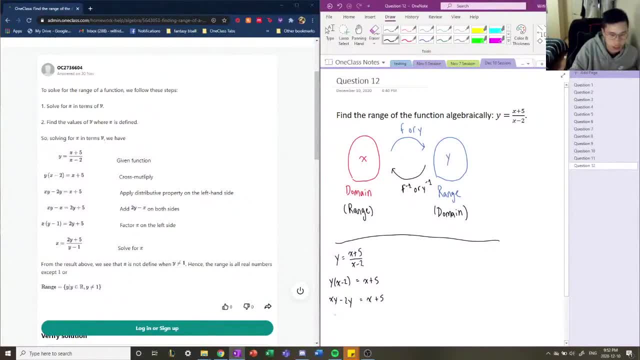 So we're going to move this 2y to the other side and move this x to this side, so we get xy minus x equals 2y plus 5, okay. And then we're going to solve for x. So we are going to factor our x and we get this. 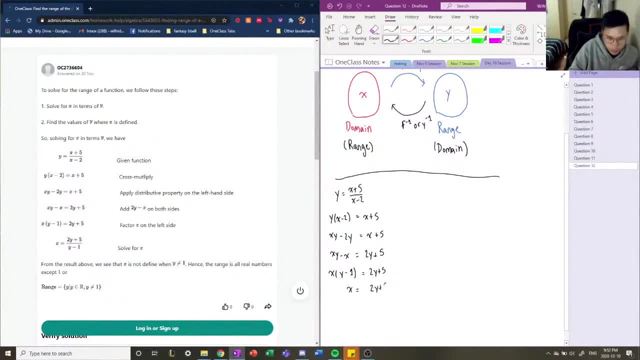 And finally we isolate and we get 2y plus 5.. Okay, so now we have found the inverse function, which is a function of y that converts it to an x value. okay, So now we want to solve for the domain of this new inverse function. right. 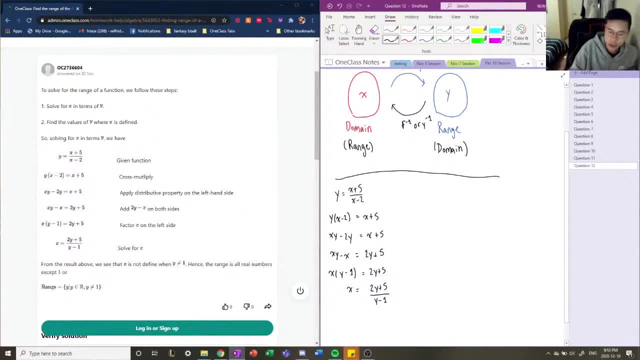 So we know that the domain of this inverse function is going to be, so we see that this is a rational function. So that means that most values of x make this, This function valid or define this function, except for y equals 1.. 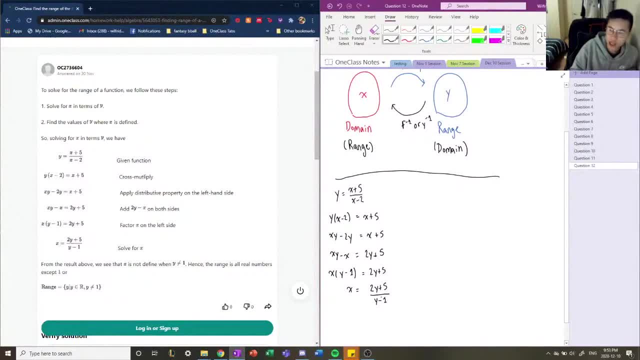 Because when the denominator is 0, then we have an undefined value. okay, So we notice that the domain of this function is y, such that y belongs to all real numbers, except for y cannot equal 1.. Okay, And this is going to be our range because, like I said, the domain of our inverse function 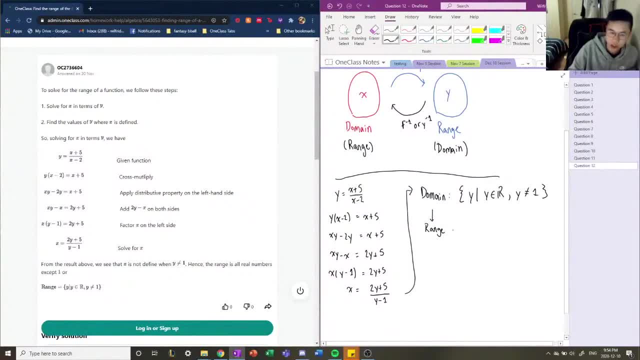 is the range of our original function and that's what we're trying to find. So this is the range of our function. Range of y equals x plus 5, 5x minus 2 is y, such that y belongs to all real numbers. 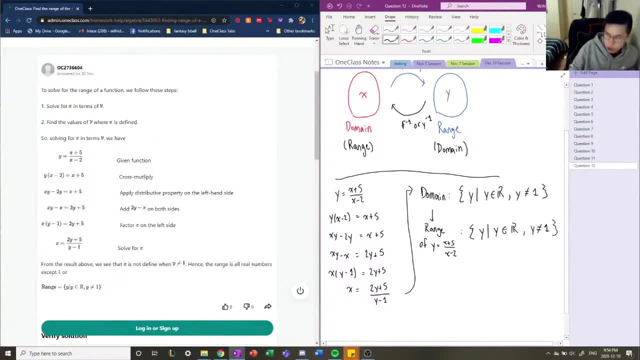 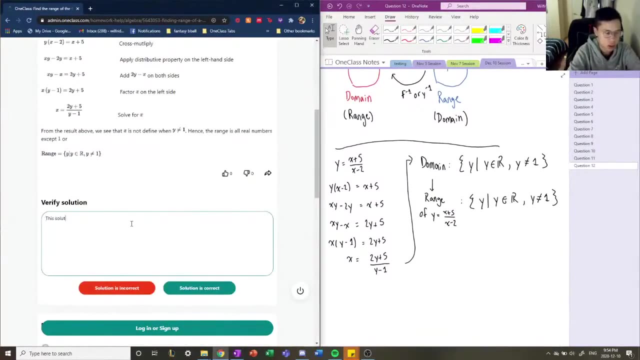 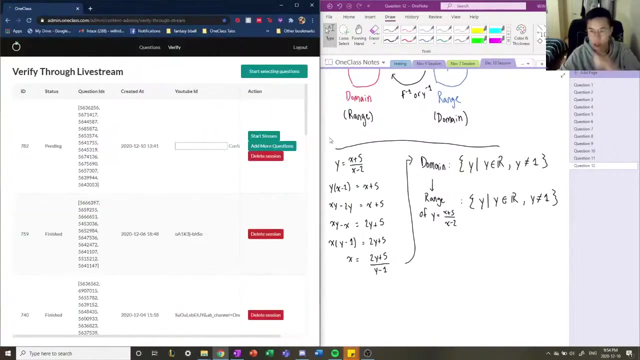 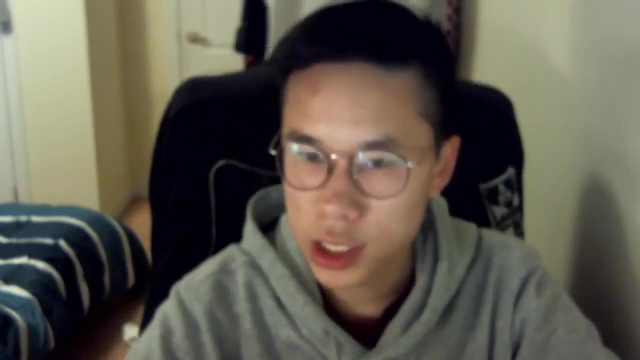 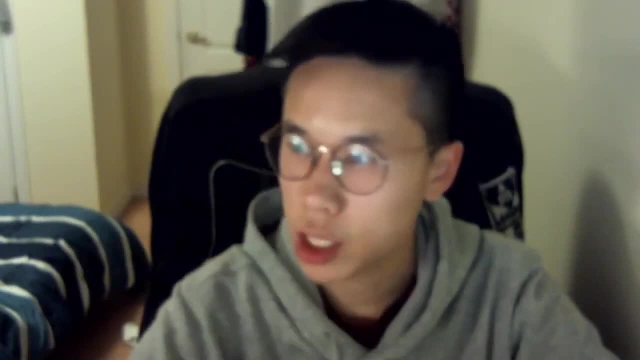 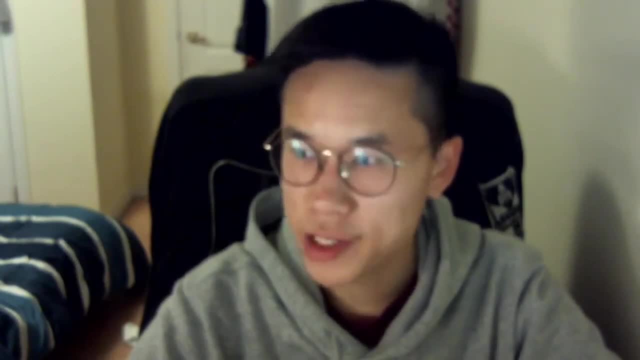 Bye-bye, Bye-bye, Bye-bye. Other than that, I wish you guys a good night and hope you guys learned something. Bye, guys.